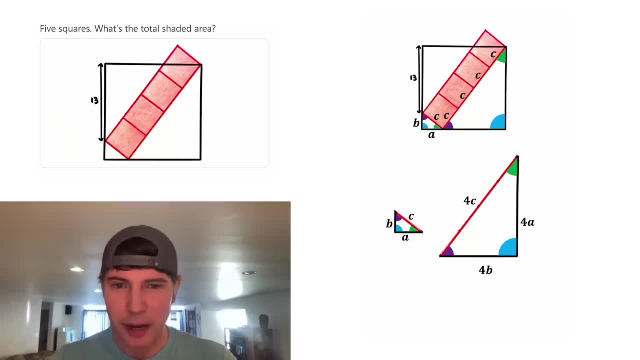 know these sides, So we can update this figure. Let's rotate this triangle back and you can see that the four B goes there and the four A goes there, So that looks pretty good. Now we have three different ways to measure the side of this larger square. Let's set them equal to each other, So. 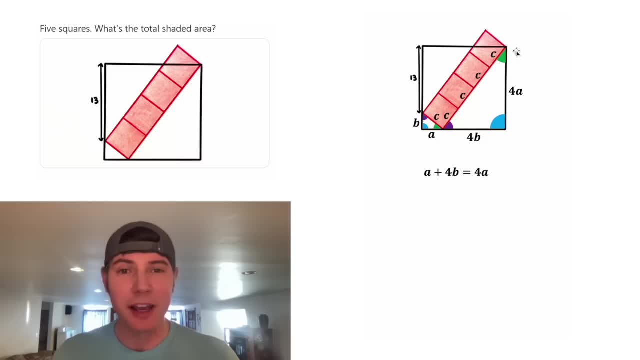 we'll have this side A plus four B, equal to this side four A. And then we can also do this side B plus 13, equal to this side four A. And now we have two equations and two variables, So we can solve for both A and B. Let's start with this one. We can subtract A from both sides and that gives us: 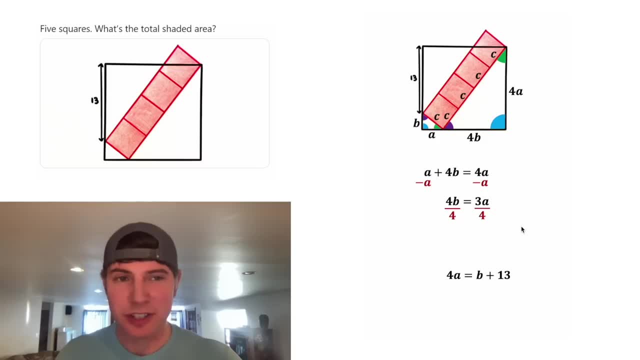 four B is equal to three A, And next we can divide both sides by two, So we have four B plus three A, And that will give us B is equal to three fourths A, And this looks important. So let's put a box. 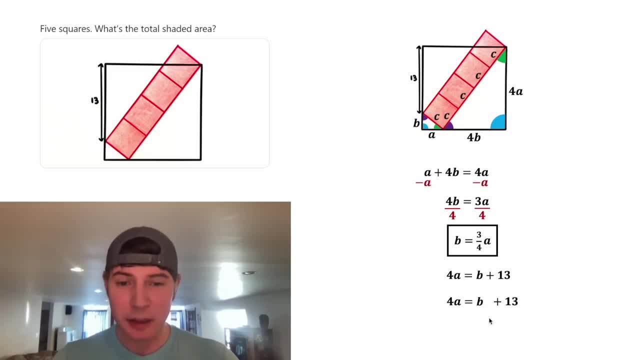 around it. Next, let's look at this equation, Let's copy it down And in the place of the B we're going to plug in three fourths A, And then we want to combine like terms. So let's subtract three fourths A from both sides of the equation. On the right hand side, these are going to cancel. 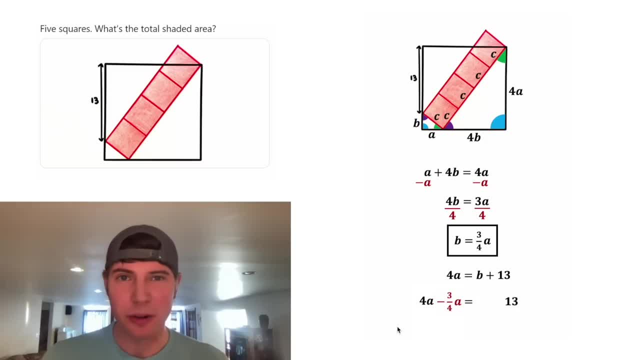 each other out, And on the left hand side, we're going to do four A minus three fourths A. In order to subtract these, let's give them a common denominator. Let's rewrite this four as 16 fourths, And then we're going to do four A minus three fourths A, And then we're going to. 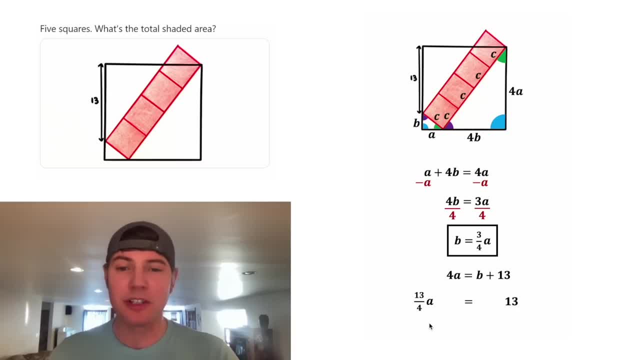 do 16 fourths A minus three fourths A, which is equal to 13 fourths A. Now to get the A all by itself, we'll multiply both sides by the reciprocal four thirteenths. On the left hand side, these are: 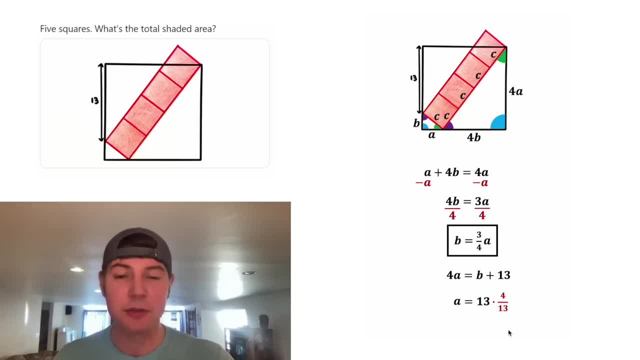 going to cancel each other out, And on the right hand side, these two thirteens will cancel each other out. So we end up with: A is equal to four, And this looks important, So let's put a box around it. Now, going back to our previous box, we know B is equal to three fourths of A. A is equal. 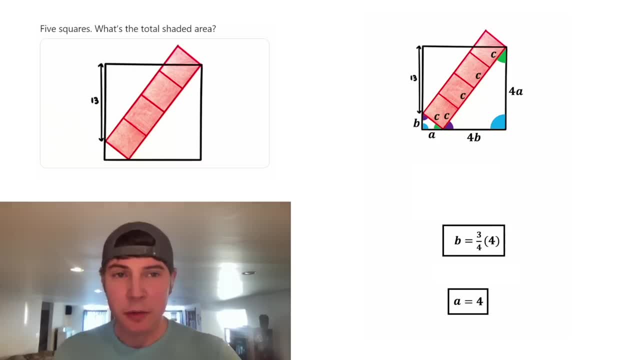 to four. So in the place of this A, let's plug in four, And then we're going to multiply both sides together And then, when we multiply this three, fourths times four, the fours are going to cancel each other out. We end up with B is equal to three. In the place of both of these A's, we can: 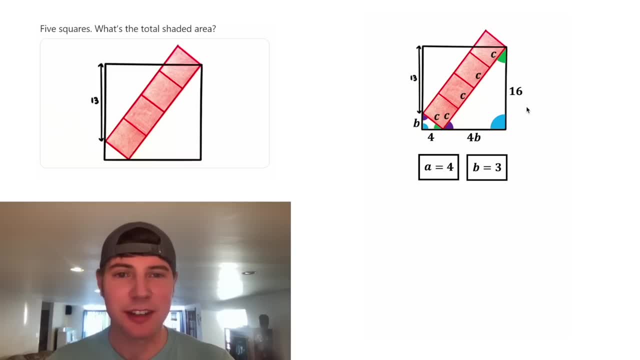 plug in four, And then four times four is equal to 16.. And in the place of both of these B's we can plug in three, And four times three is equal to 12.. So now let's focus on this little triangle.